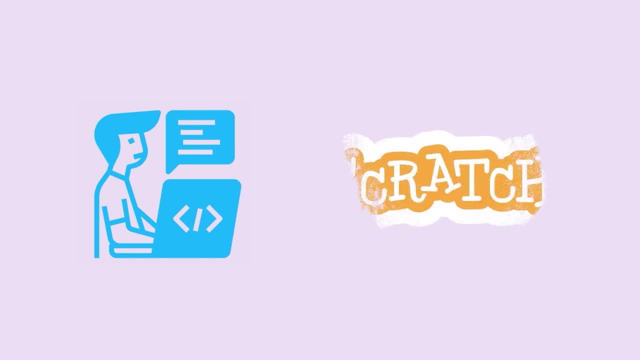 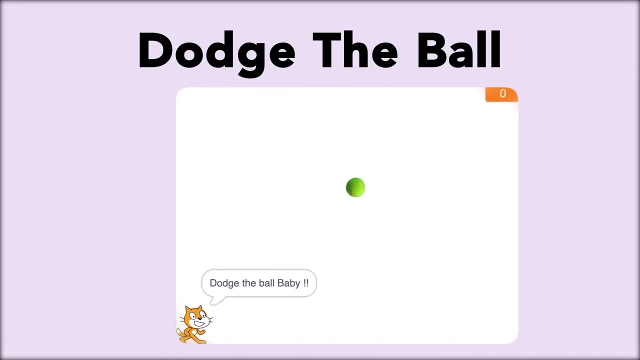 and that was the first time he came across this programming tutorial called Scratch, where he wrote code for the first time and built a game called Dosh the Ball, and here is how this game looked like. I know you would be confused as to how flyweight pattern and this scratch game. 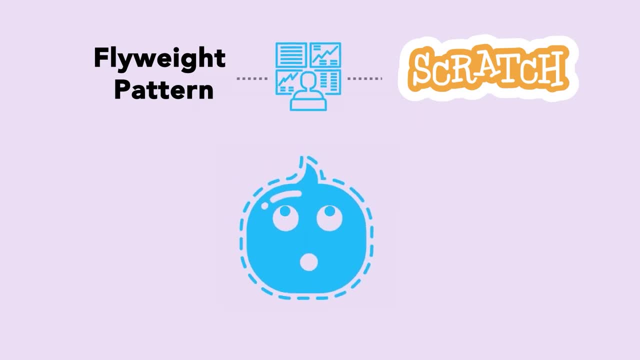 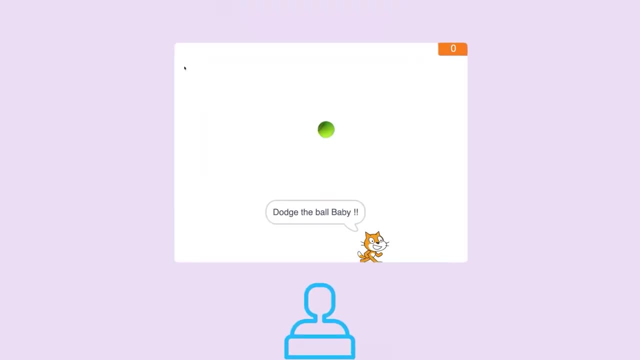 have to do with each other or, this day, stock trader. but just stay with me for one minute and I promise all of this is going to converge. The trader built this game and was very happy playing this game, crossing one level after the other, but as the number of levels increased. 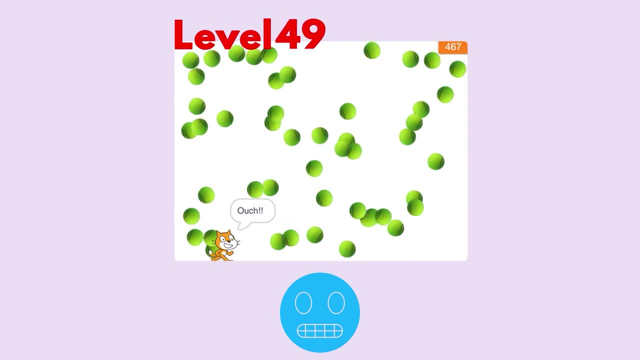 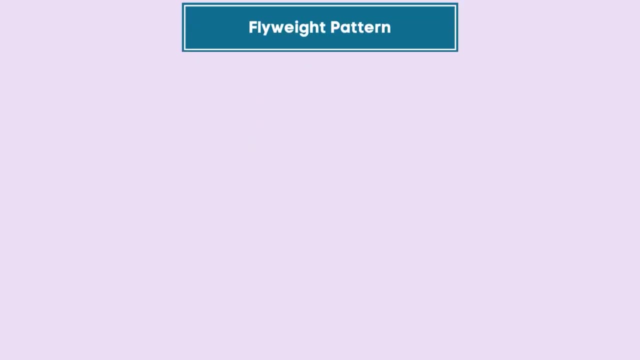 the number of balls also increased and the game eventually slowed down. Little did he knew that he could have used this game to make money, So he started a new game called Dosh the Ball, and he used flyweight pattern to optimize this game. So there it is: Flyweight pattern is an 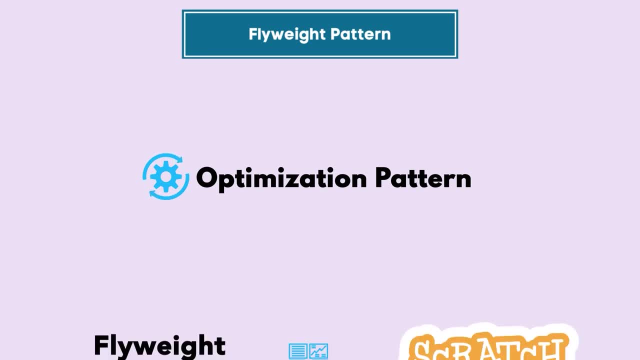 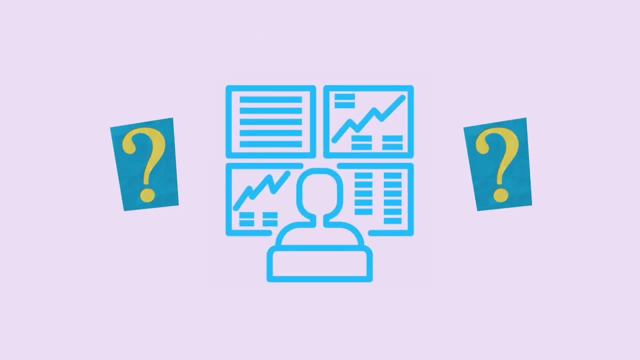 optimization pattern. See, I told you it will all converge. Now let's get into the details of flyweight pattern. and yeah, about that trader. I will tell you what happened to his career towards the end of the video. Flyweight pattern, being a structural pattern, is actually an optimization. 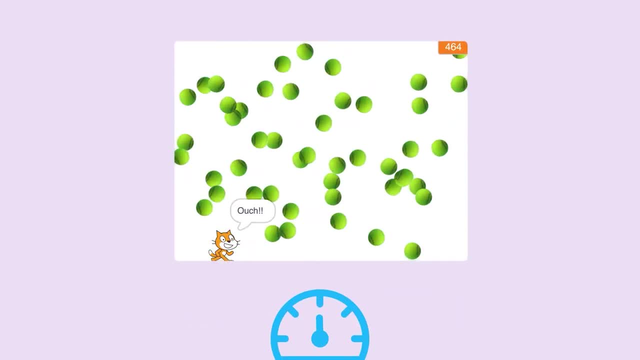 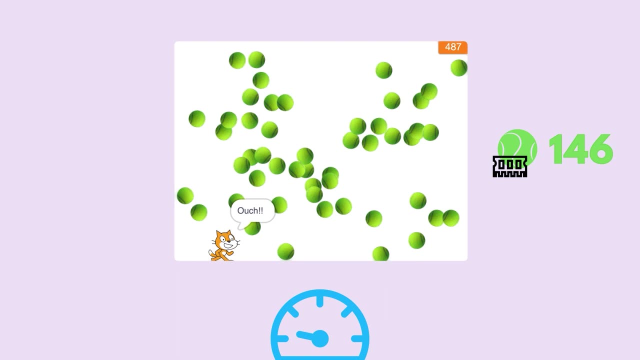 pattern and the game that we just looked at slowed down because of the increased number of balls, started using a lot of RAM. So the game slowed down because of the increased number of balls and hence using flyweight pattern. could have solved that? How flyweight pattern would have. 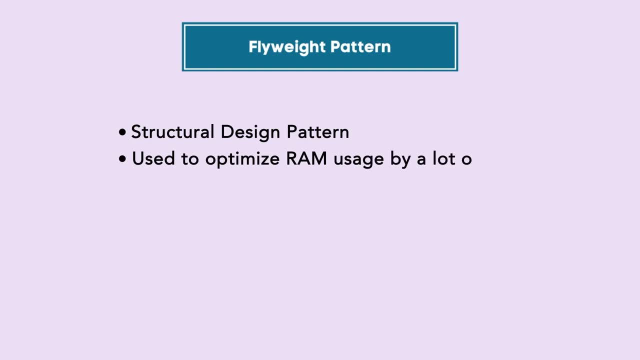 solved that Because it is used to optimize the RAM usage by a lot of objects which share some immutable state. Some examples of flyweight pattern, or some examples where flyweight pattern can be applied, are car games with a lot of repeating objects or trees, etc. or e-commerce app listing. 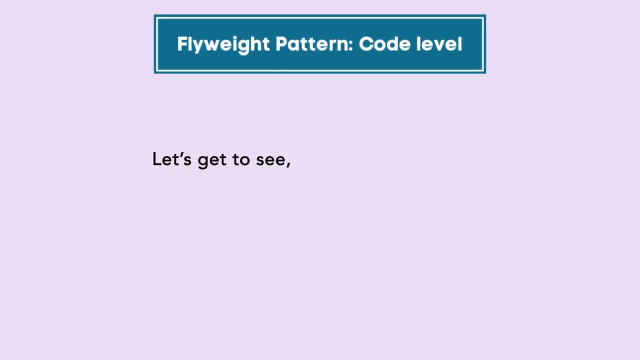 and selling thousands of items. Now let's get to see at the code level that what happens in a flyweight pattern, So here it goes. So let's get to see at the code level that what happens in a flyweight pattern, So here it goes. In the above dodgeball example game you have seen that there. 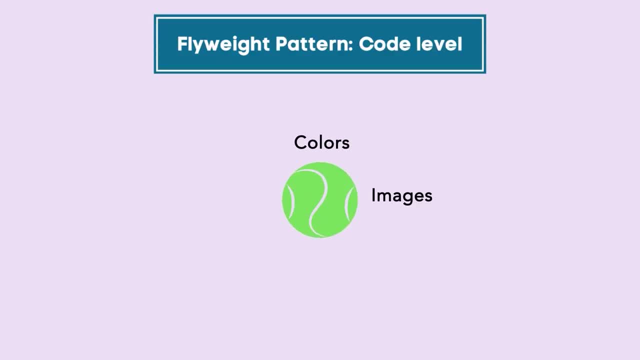 was a ball object and it has properties like color images, coordinates, x, y, radius of the ball, and so on. The functions for this class would be to draw the ball on the canvas. The properties, which would not change with more number of balls or the more number of instances of the balls, are color or 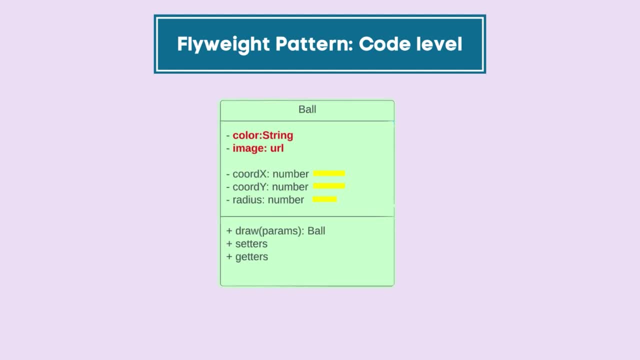 image. The properties that would change are coordinates or radius. These properties, which do not change, are called intrinsic attributes. However, the properties that would change are called extrinsic attributes. Every time a new object is initialized for this class. these properties remain same, But the extrinsic properties over here do change Every time a ball object is. 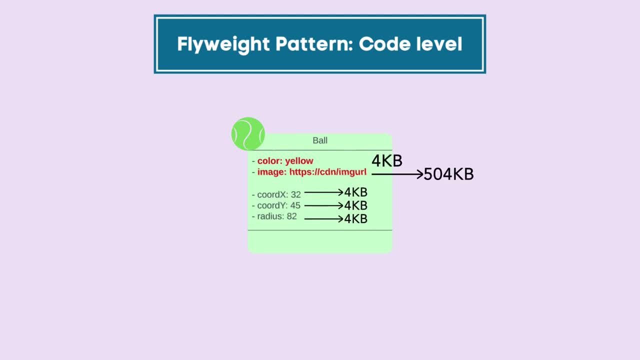 initialized, some memory is needed for that object during runtime, including intrinsic and extrinsic properties. Approximately 504 KBs of memory is required for one object, And when we get to a case where we have to have hundreds or thousands of these objects, we have to have a number of objects. 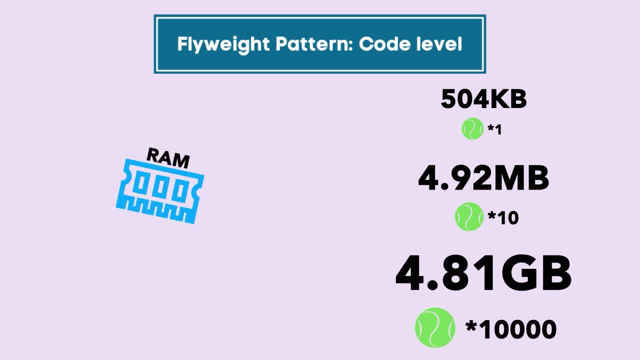 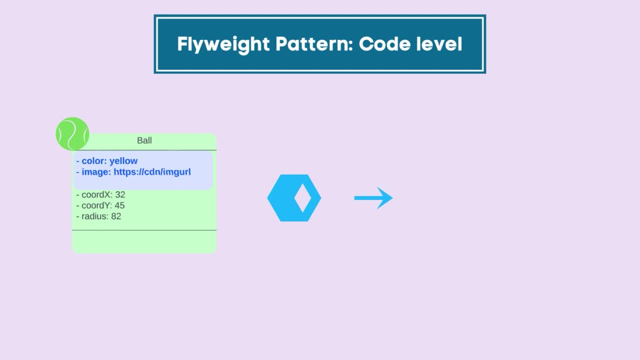 and we can see how the memory increases or the memory usage increases. In reality, we can extract out these immutable properties or intrinsic properties of these objects, like color and sprite, in a separate object, and we can reuse these abstracted out objects. All we have to find out. 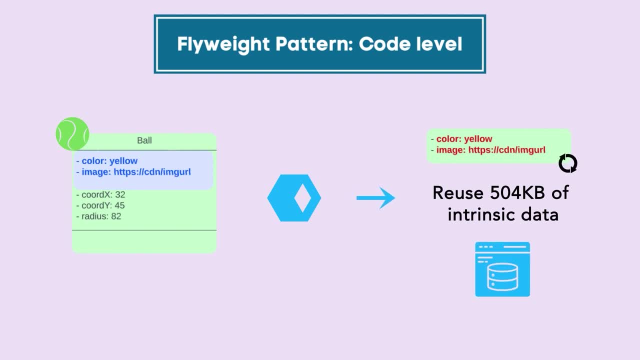 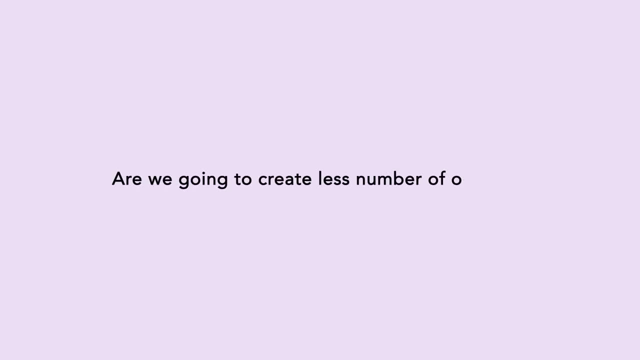 a way is to store them and cache them somewhere in the application, And hence we would be able to save a lot of memory. You would wonder that if we are going to save a lot of memory, are we going to save the number of objects? No, the number of objects still remain the same, except the data. 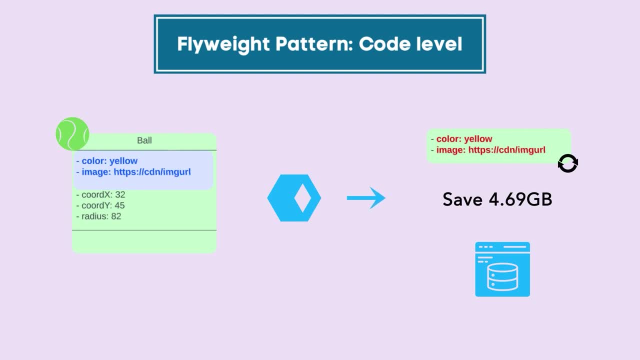 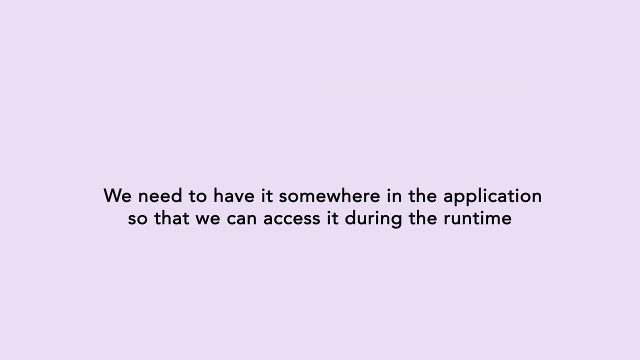 which takes a lot of memory and is common among all the objects, is extracted out. Now the question is the extracted out data. where do we save that data, or where do we save that object? We need to have that stored somewhere in the application so that we can access it during the runtime. So 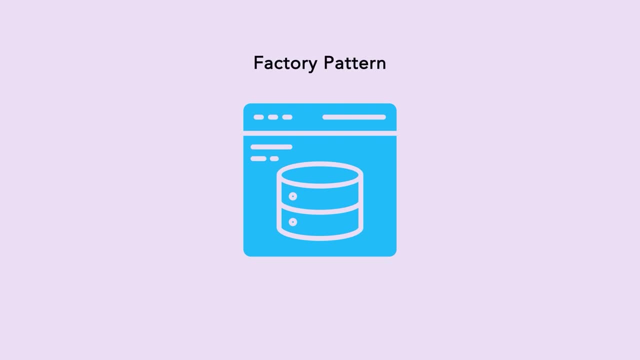 we cache that intrinsic data using a factory pattern, and those objects that we cache using a factory pattern are actually known as flyweights. Here is a visual representation of a flyweight. The flyweight is a pattern of how the objects and the memory usage would look like before. 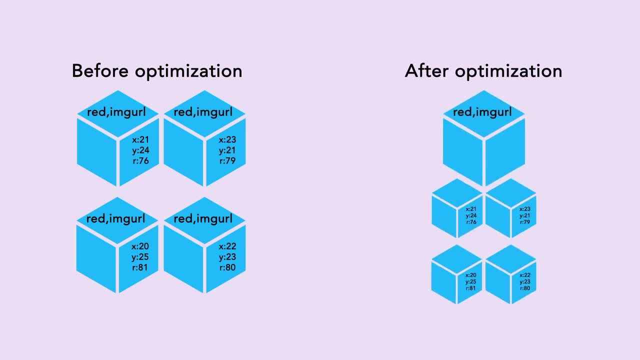 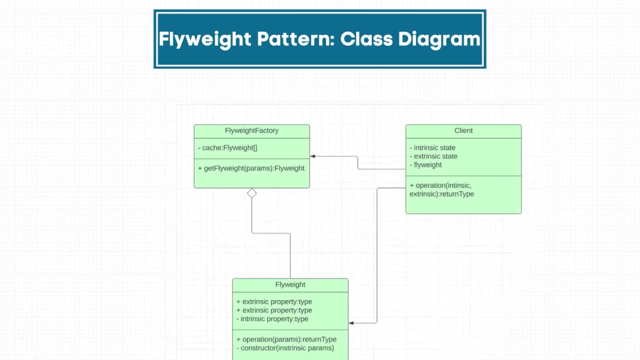 optimization and here how the objects are going to look like after the optimization. The class diagram for this pattern can be a bit tricky, but let's try to take a dig at it. You would use a factory pattern to cache all the flyweight objects in an array, Your flyweight. 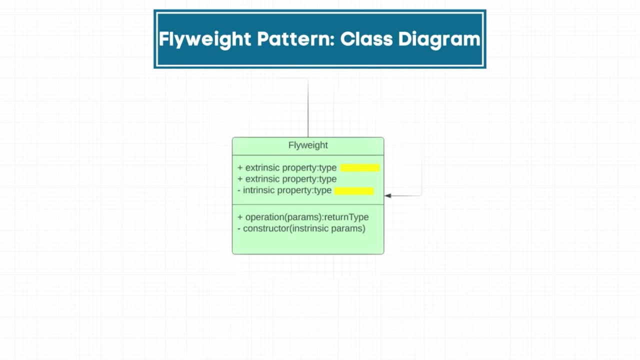 object is going to have intrinsic and extrinsic properties. The flyweight factory is going to cache the objects. If that object has already been created, it will return that same object And the client that is using this code will use the extrinsic properties to further enhance. 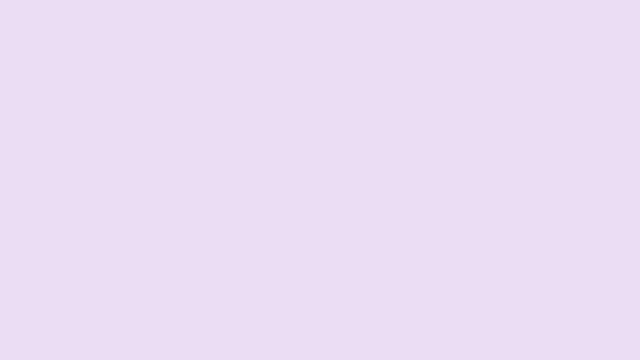 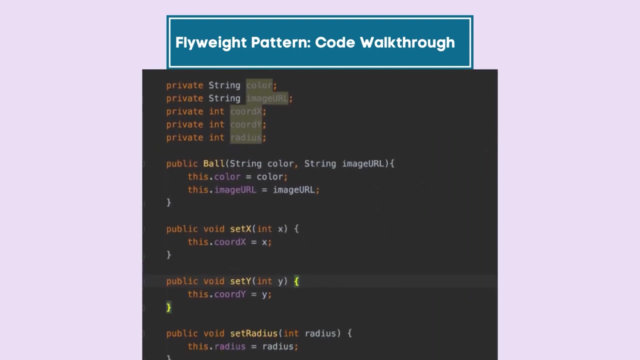 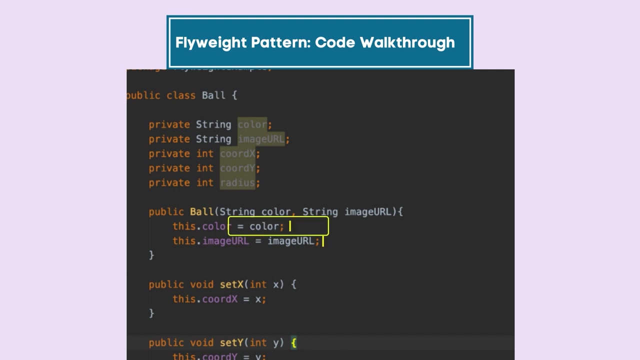 that object and further use it in implementation. Let's try to look at concrete code to understand this. This is the ball object that we had been talking about. It has all these properties that we have just seen. What we have done here is that we abstracted out colour and image URL and made it a part of the constructor. 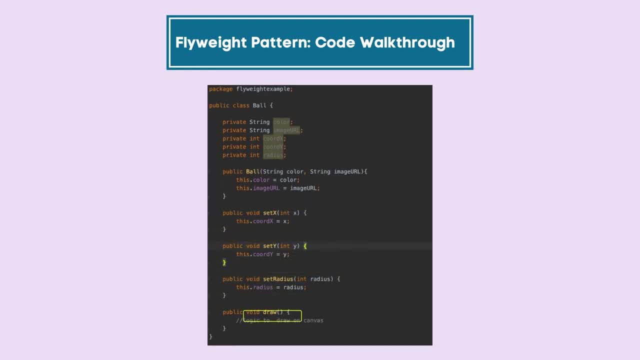 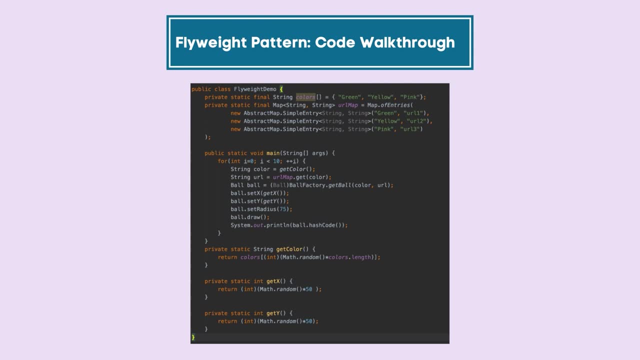 The other properties have their setters and a draw function for this ball, But colour, old and image URL do not have external setter functions. This is our main client code which is going to use the flyweight factory and the flyweight pattern. So as you can see here that we have 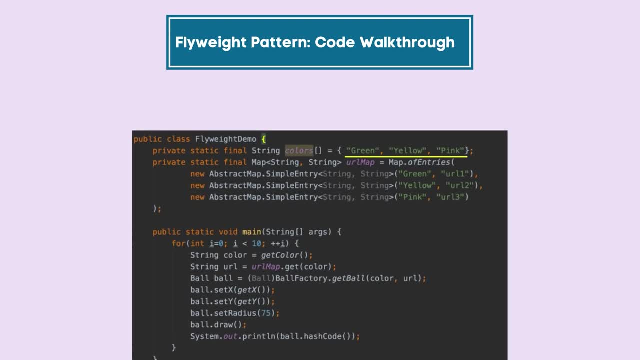 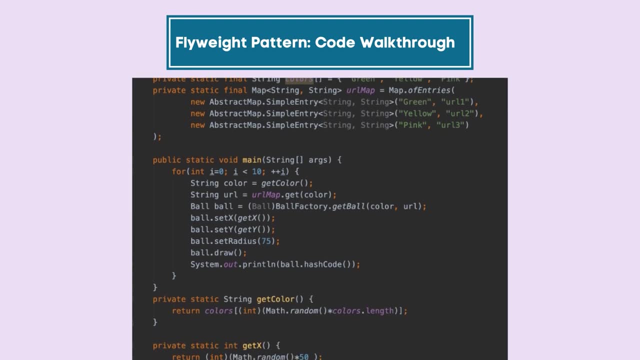 some different colors using which we can initialize different color balls. We have created a map using which which color ball has a respective image URL. Now, as you can see here in this particular piece of code, we are trying to get the color, the respective image, and we 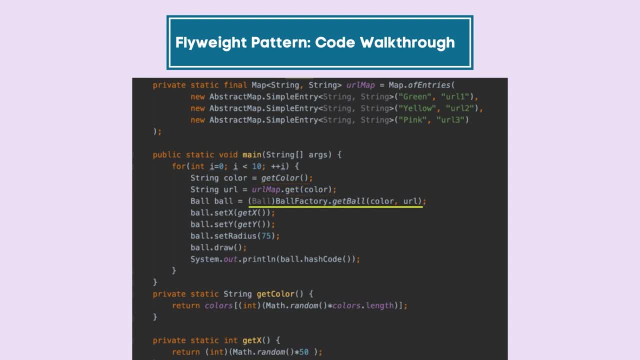 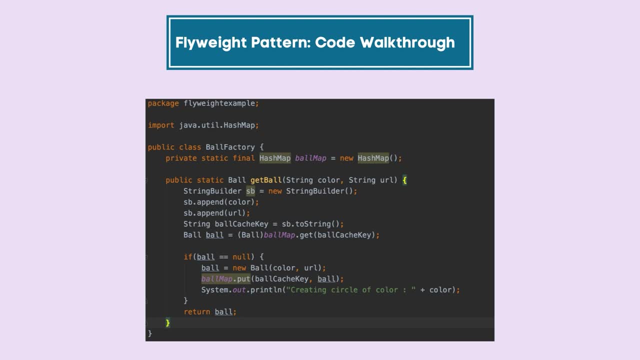 are trying to use a ball factory to get the ball object. Now let's try to go to the ball factory class and see what's happening there. In the ball factory class, as you can see that we are getting the color and URL and on the basis of these two properties we are checking. 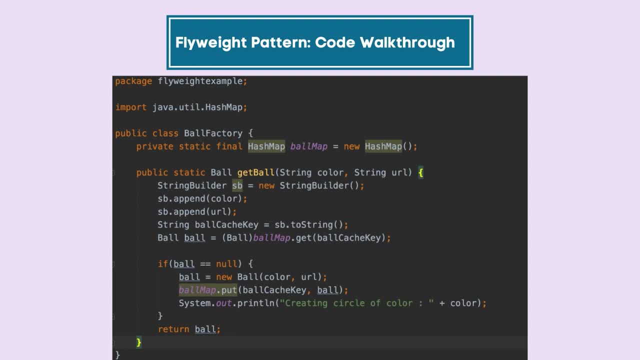 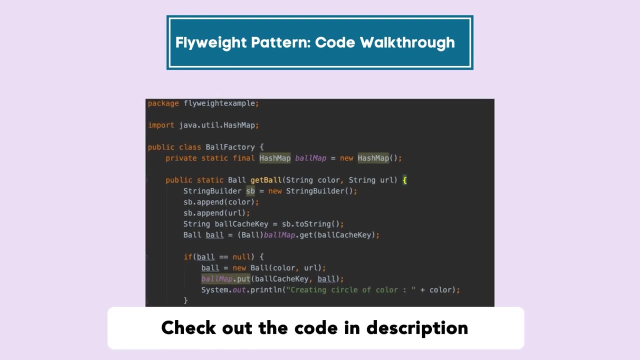 if we have something in our cache. If we don't, we are creating a ball object using those two properties and we are inserting it in our hash map- or cache for that matter- and then returning it. In case we already have that object, We will just return it from the cache. I have also added this code in the description, so 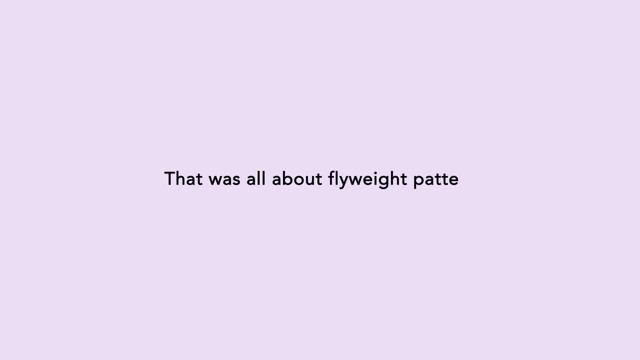 you can refer it at ease. So that was all about flyweight pattern. Now let's go through some pros and cons. The obvious pro of this particular pattern that it is an optimization pattern and it's very useful to save the resources. Some cons would include that there is a factory. 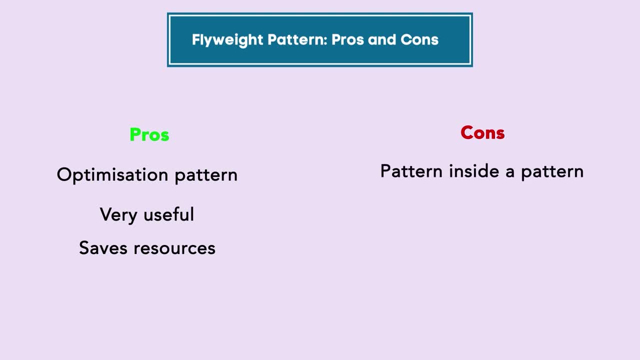 pattern and there is a flyweight pattern, so there is a pattern inside the pattern and hence it can be complex to understand. Sometimes it can also be a trap for premature optimization, So please make sure that you don't fall in this trap and you only use it when it is absolutely necessary. If only this stock.